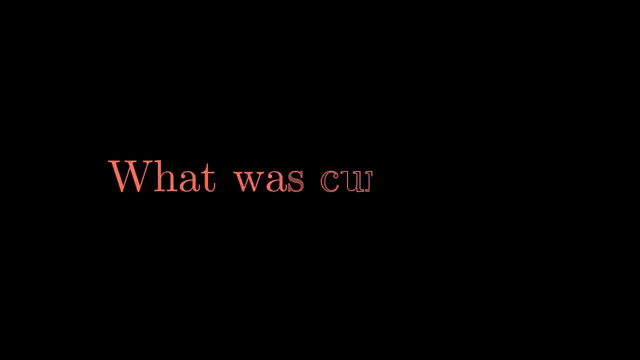 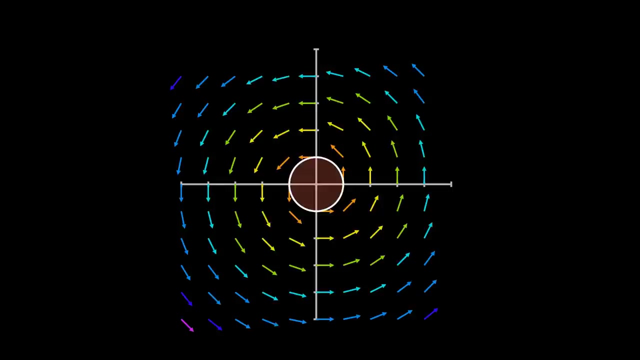 the two-dimensional curl of F over R. The curl of a vector field in two dimensions gives a sense of rotation over a region in the vector field. The curl of a vector field can now describe how clockwise or counterclockwise the region is. Positive curl indicates counterclockwise rotation. 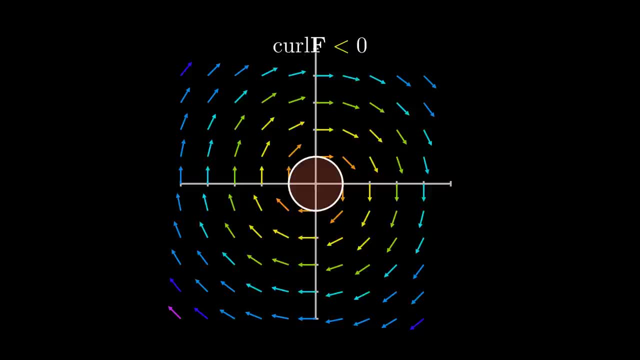 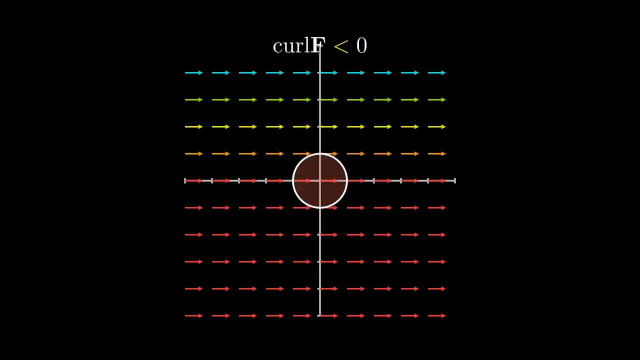 and likewise negative curl indicates clockwise rotation. Non-zero curl doesn't always occur in vector fields that look like circles. For example, we have a region with higher magnitude vectors on the top and lower magnitude vectors on the bottom. This results in an overall clockwise rotation which is negative curl We can represent. 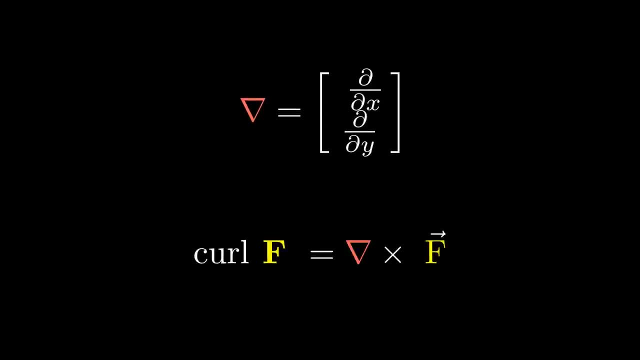 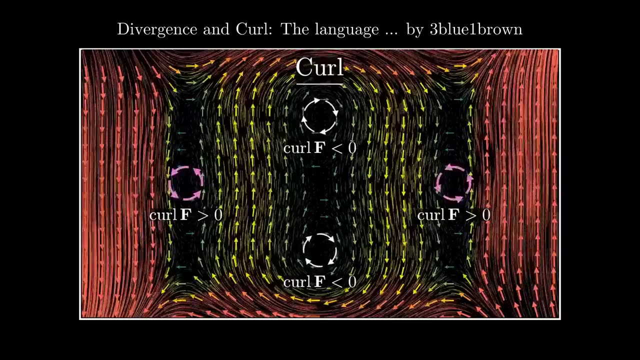 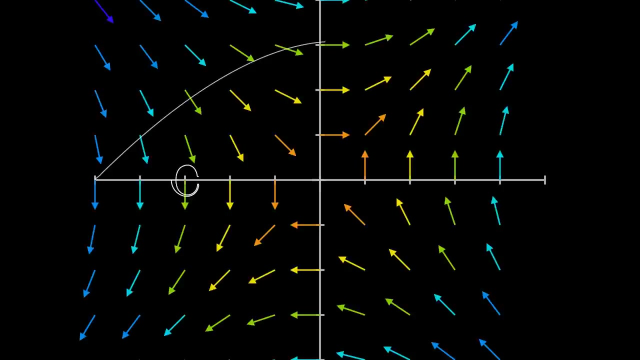 curl as a cross product between the del vector- which, by the way, is every partial derivative- and the vector field. For now let's not go over why, but I highly suggest watching this video by 3blue1brown if you're curious. First let's look at the line integral of our vector field. Here's the important bit. If the overall 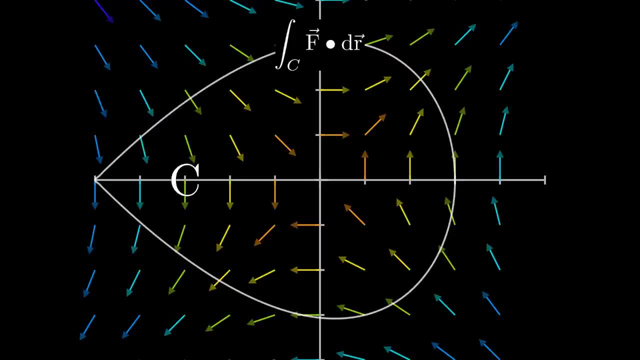 rotation of the region R is counterclockwise. the line integral will be positive and negative if the overall rotation is clockwise. Now let's look at our line integral. What would happen if we split it into two curves? The resulting integral is the line integral of F over C1 added. 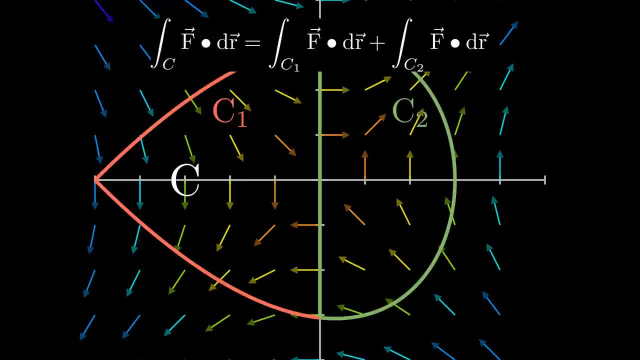 to the line integral of F over C2.. If we look at this, it's the same as the line integral over C. This is because the center line cancels out. One is going from up to down and the other one is going from down to up. This is a really important fact. 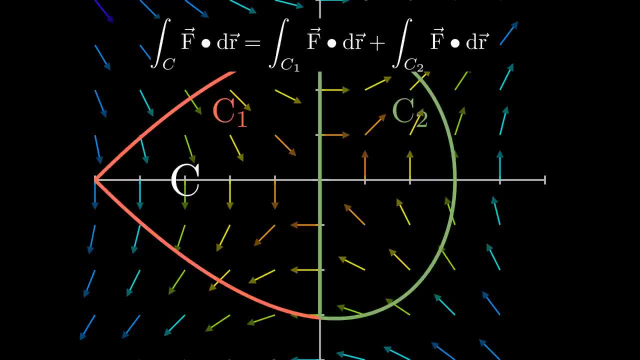 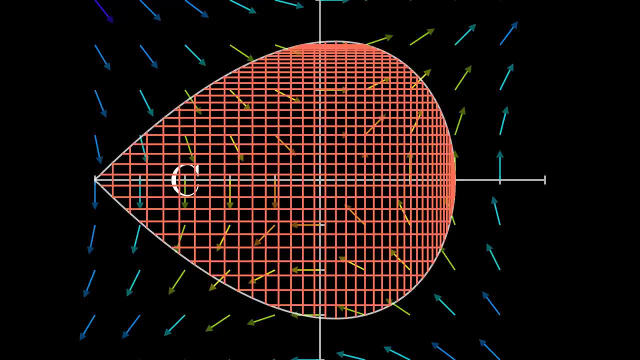 It means that we can split our curve into any amount of curves and, as long as they add up to the same curve, we can add the line integrals together and get the line integral of the outside curve. Now let's split our region into many, many small regions, If you. 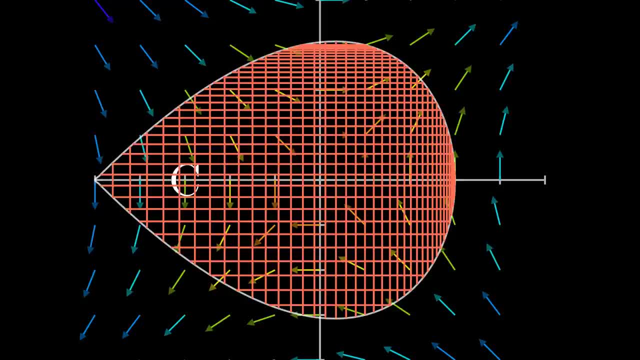 all. we have another way of describing rotation of a vector field: curl, As we described. curl is for points in a vector field, So we can approximate our line integral by summing up the curl times: a small region for every single point on our region. This is just a. 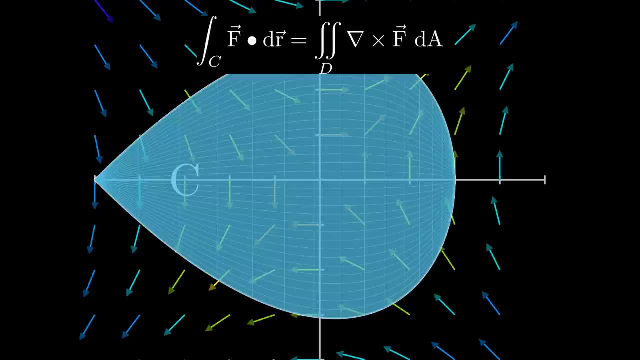 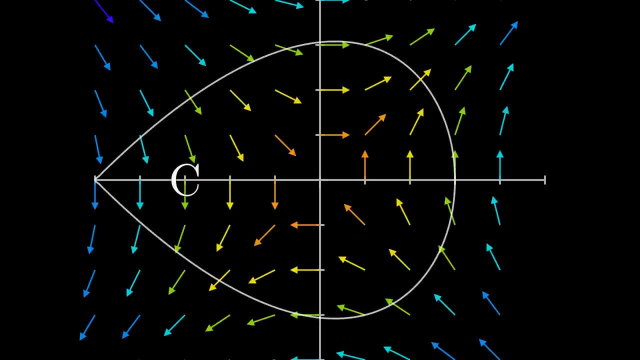 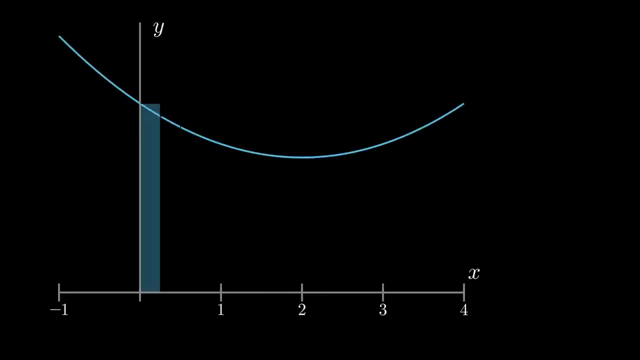 double integral. Let's go over that again. In calculus, we always use this idea of using infinite approximations. For example, we did this when learning about the definite integral Using Riemann sums. the area under a curve was approximated and the integral was the. 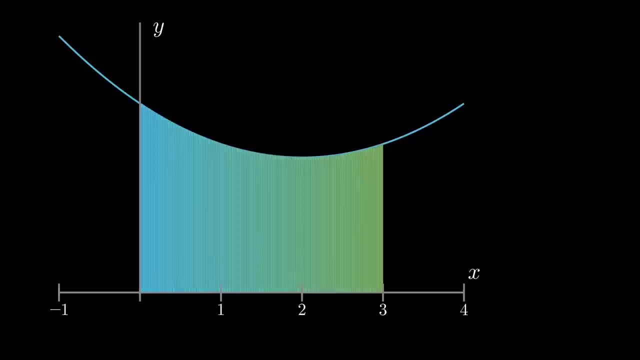 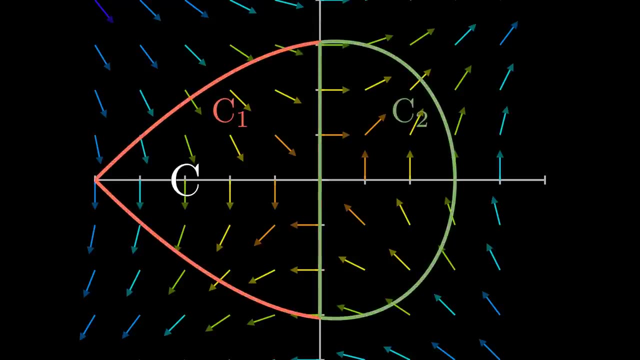 sum of these areas as we approached infinite number of rectangles. In the beginning we established that we can split a curve into as many pieces as we want and sum up the line integrals of each of these pieces to get the line integral of the whole. 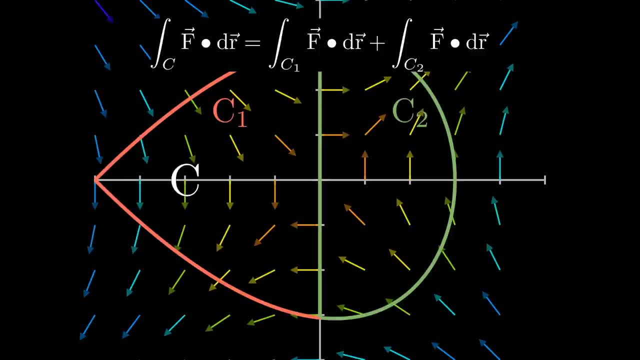 curve. In a calculus sense, we might see what happens when we use the integral as a sum of the sum of the line, integrals of the whole curve. In this case, we use a ton of more rectangles As the size of the rectangle approaches zero. 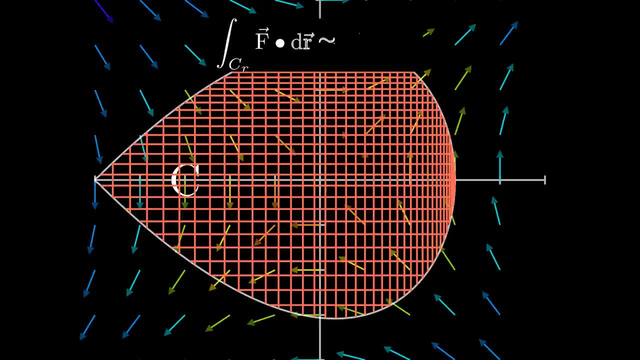 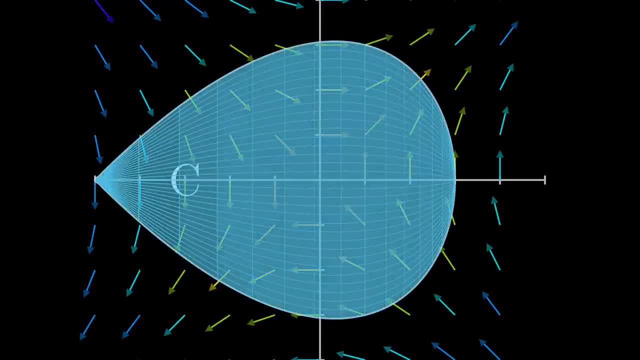 the curl of the vector field becomes a much, much better approximation for the line integral of each of the small pieces. Thus we can sum up the curl of every point inside the region of R to get the line integral of the whole curve C. If it still sounds confusing, I've left a few links in the description to articles that 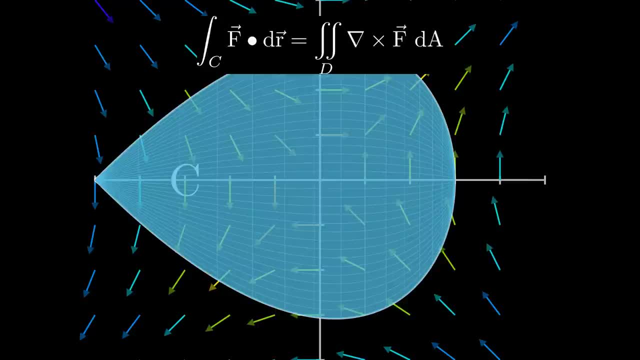 talk about this. We see this kind of approximation into equality all over calculus. It started with limits and how to get the line integral of the whole curve C. If it still sounds confusing, I've left a few links in the description to articles that talk about this. We see this. 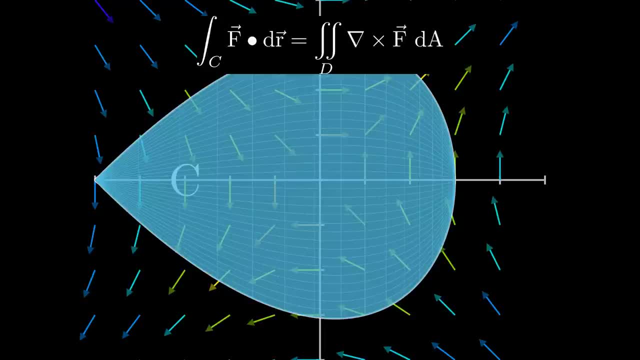 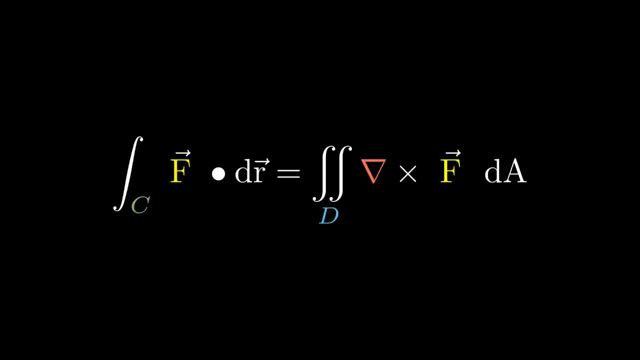 kind of approximation into equality all over calculus. It started with limits and how a function can approach a value. This is essentially the same thing. Now we have the line integral of our vector field, described as the double integral of the curl of the same vector field. This should make complete sense. What's really interesting? 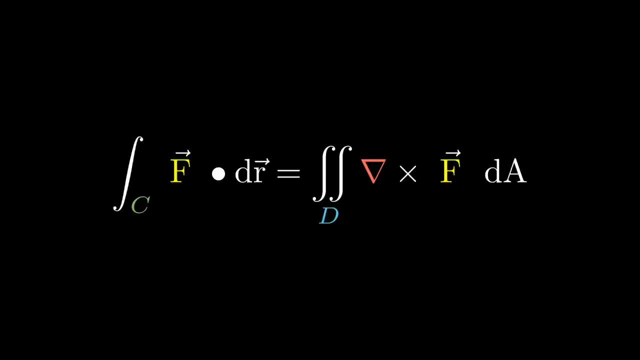 is that the double integral, which is related to the region inside the curve, can only be described that by looking at the edges. This is analogous to the fundamental theorem of calculus from single variable calculus. If you remember, this states that the area under a curve can just be described by looking 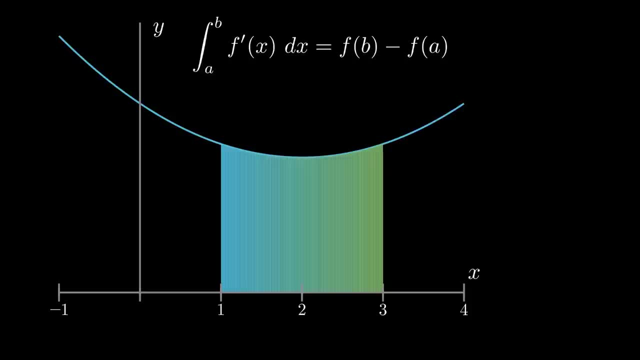 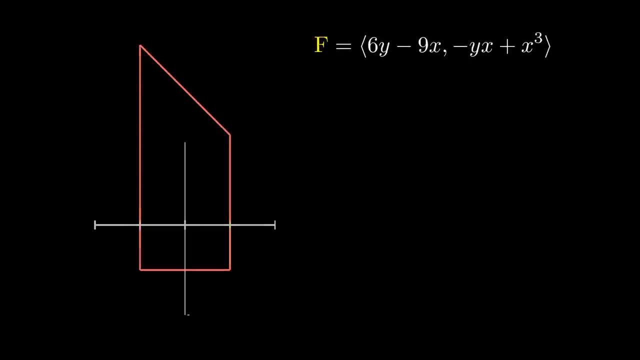 at the endpoints. Similarly, the region inside a curve can be described by just looking at its edges. Now let's look at an example of how this can be used. Let's say we have a vector field. f is equal to 6y minus 9x and minus yx plus x, cube And the curve, C is the curve.